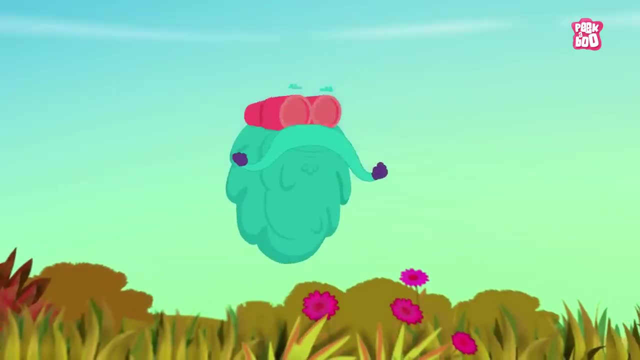 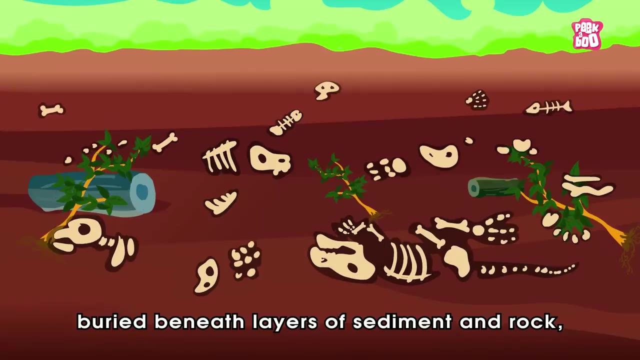 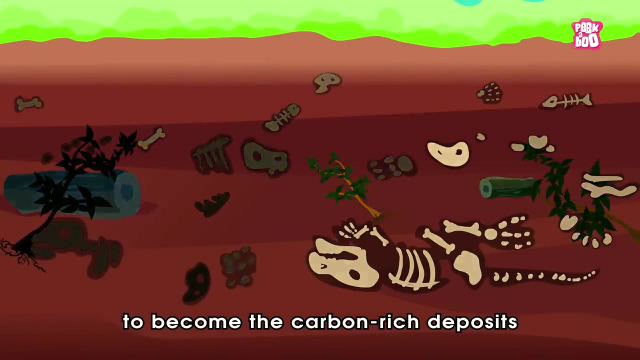 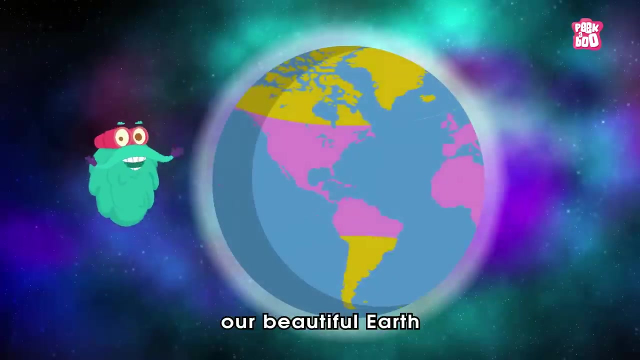 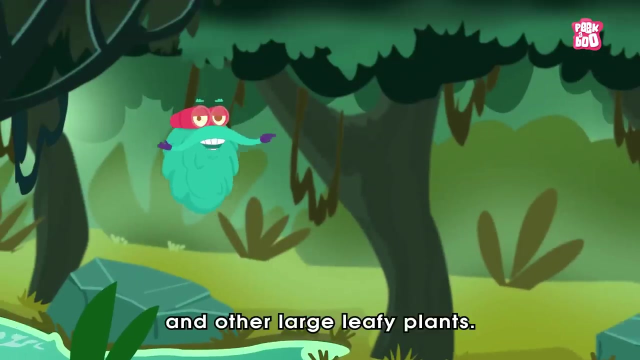 So zoom in. What are fossil fuels? Decomposing plants and other organisms buried beneath layers of sediment and rock have taken millennia to become the carbon-rich deposits we now call fossil fuels. You see, a long time ago our beautiful earth was covered with swamps filled with various microorganisms, trees and other large leafy plants. 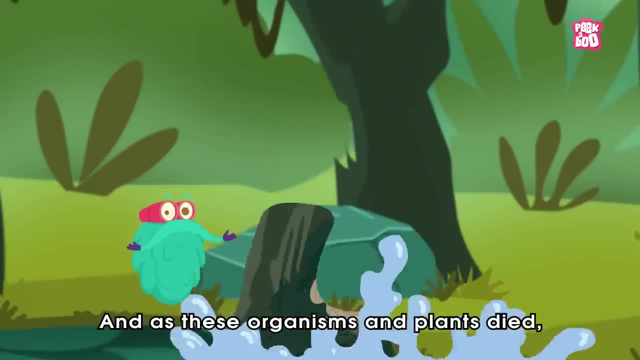 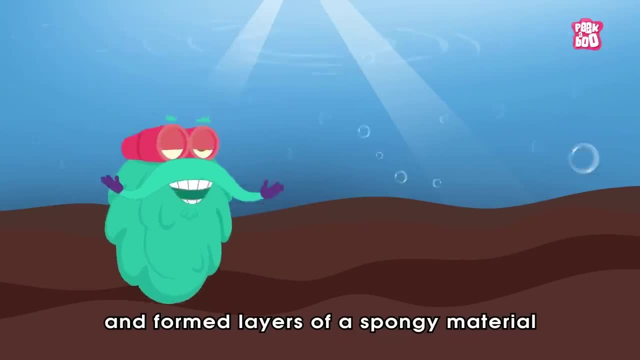 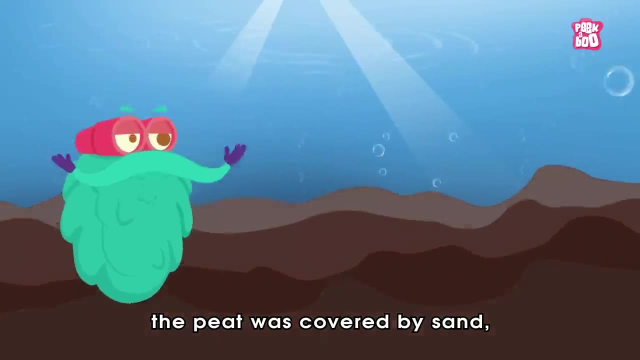 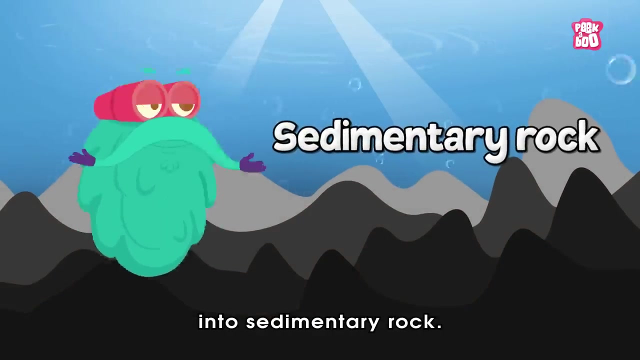 And as these organisms and plants died, they drowned to the base of the swamps and oceans and formed the earth, And they formed layers of spongy material called peat. Over millions of years, the peat was covered by sand, clay and other minerals, which converted the peat into sedimentary rock. 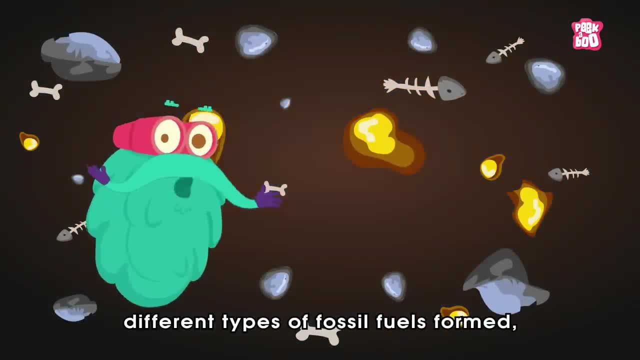 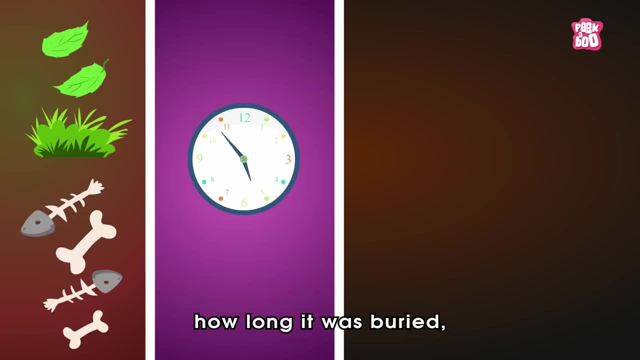 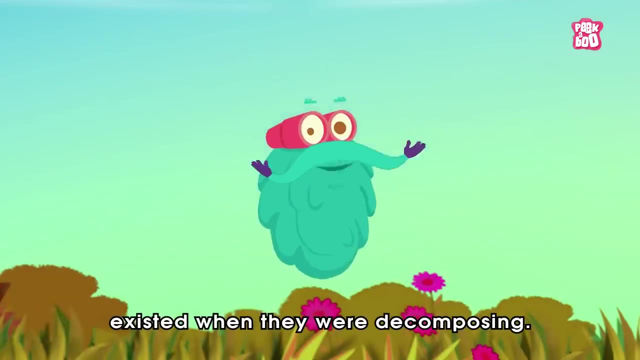 Then, over the next few years, different types of fossil fuels formed, depending on the combination of organic matter present, how long it was buried and what temperature it was in, The temperature and pressure conditions existed when they were decomposing. And what are these types of fuels? 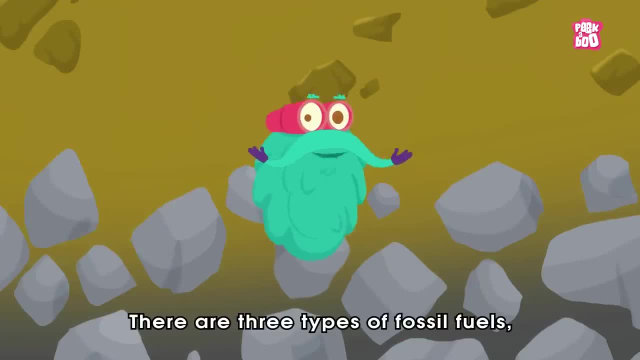 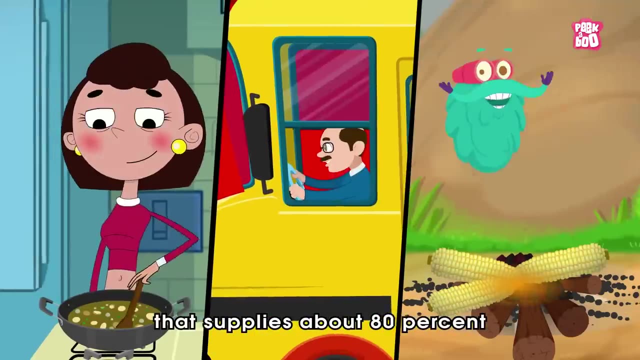 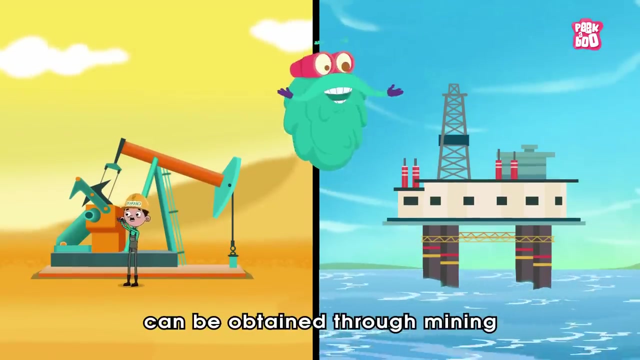 Well, there are three types of fossil fuels, namely coal, mineral oil and natural gas. that supplies about 80% of the world's energy. These non-renewable fuels can be obtained through mining and extraction inside the land or huge oceans. 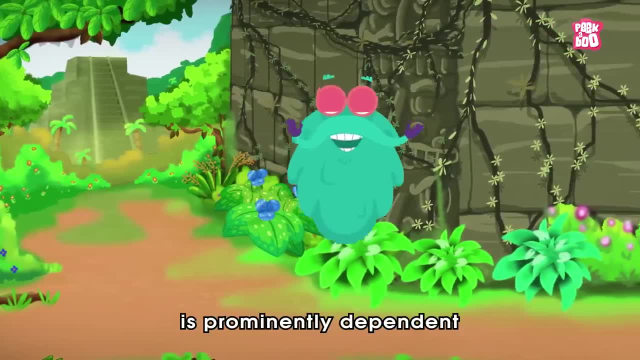 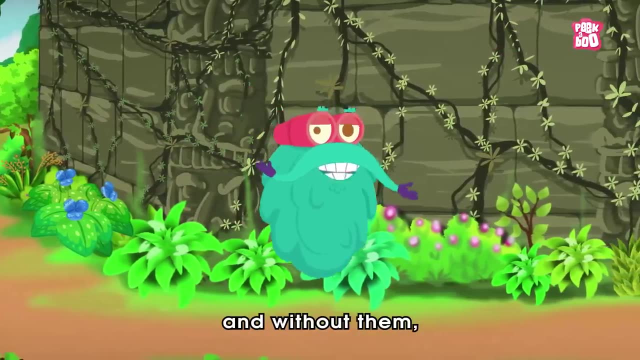 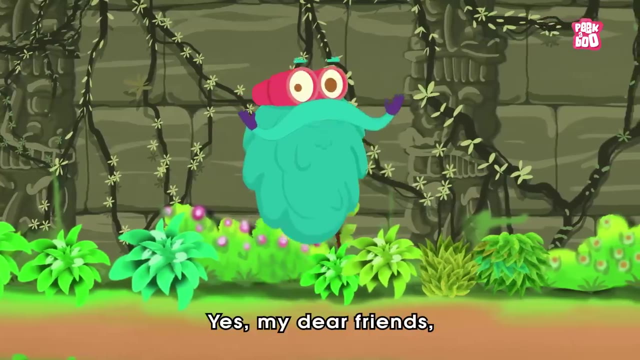 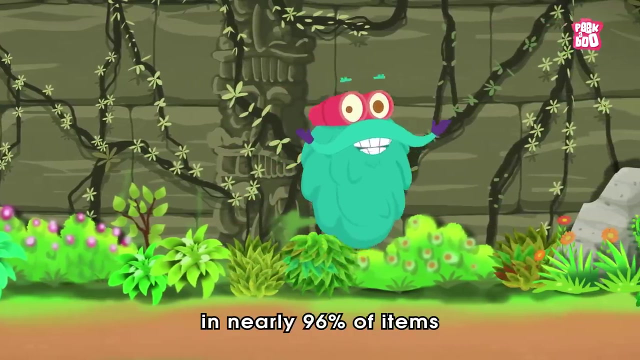 It is said that our whole human race is prominently dependent on these fuels to carry out the tasks for their existence, And without them it would be difficult for us to coordinate our survival efficiently. Yes, my dear friends, that's because fossil fuels are utilized in nearly 96% of items that we use today. 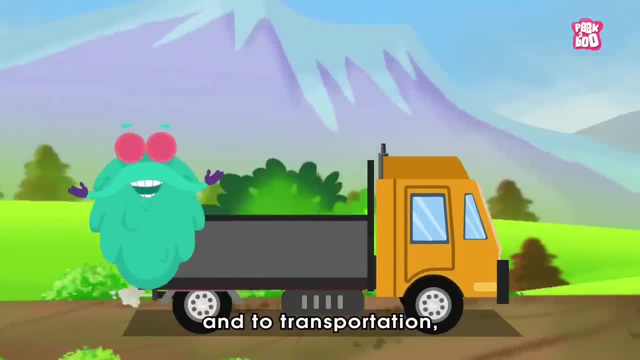 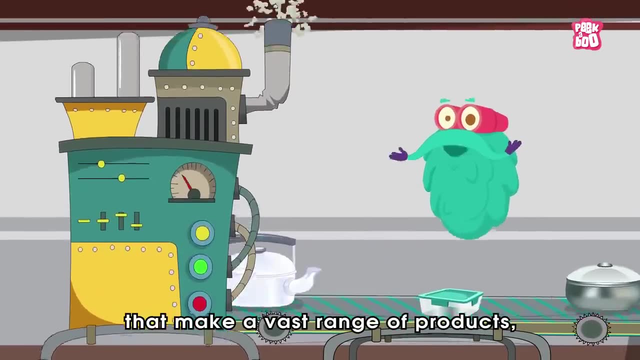 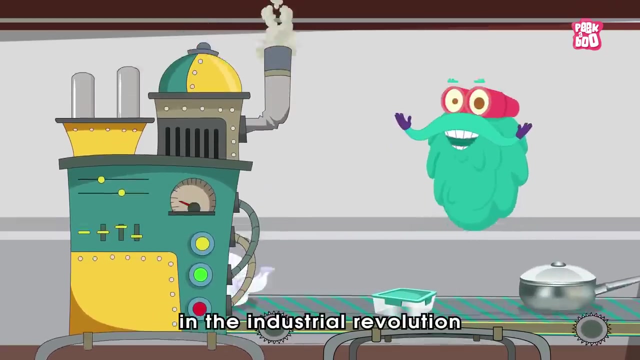 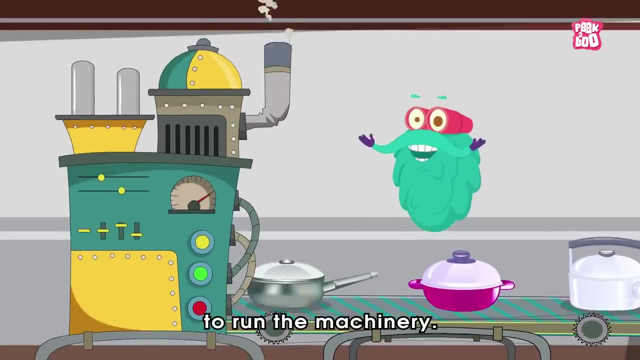 Right from the electricity to heat and to transportation, while also supporting the processes that make a vast range of products, from steel to plastics. And it also played a considerable role in the industrial revolution by providing the necessary fuel needed to run the machinery And as a dependency on these fuels. 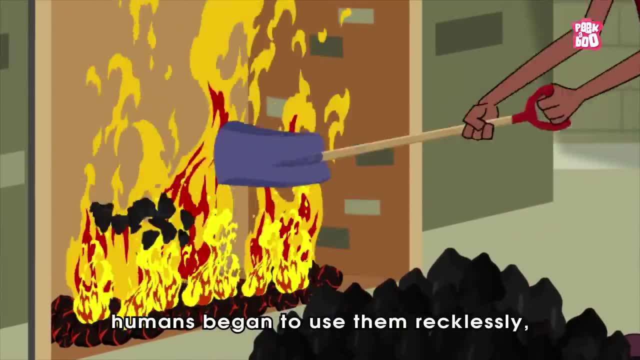 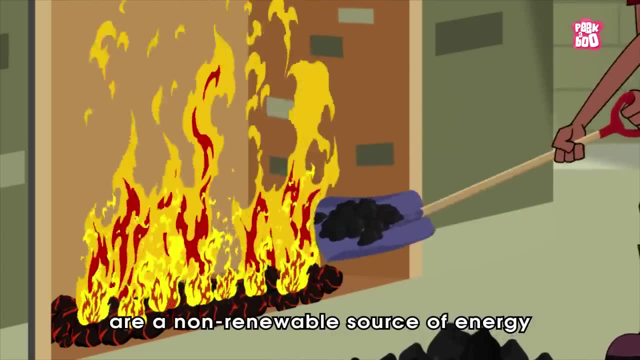 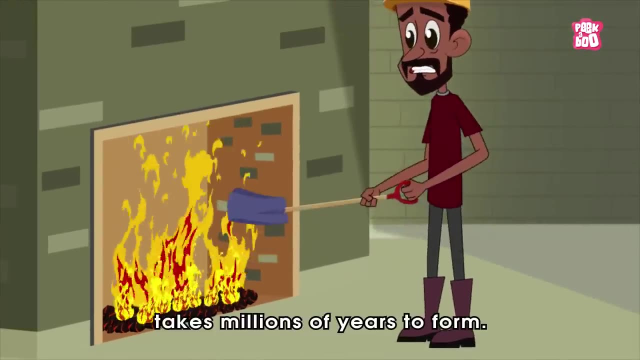 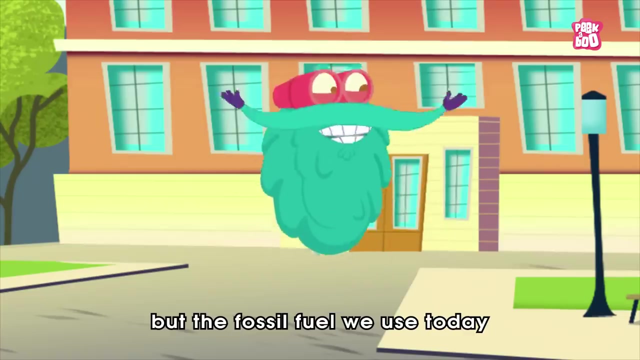 and as fossil fuels kept on increasing, humans began to use them recklessly, without considering that these fuels are a non-renewable source of energy which does not develop in a day or two, but takes millions of years to form. Yes, my friends, I know it's hard to believe, but the fossil fuel we use today started creating from the Carboniferous period. 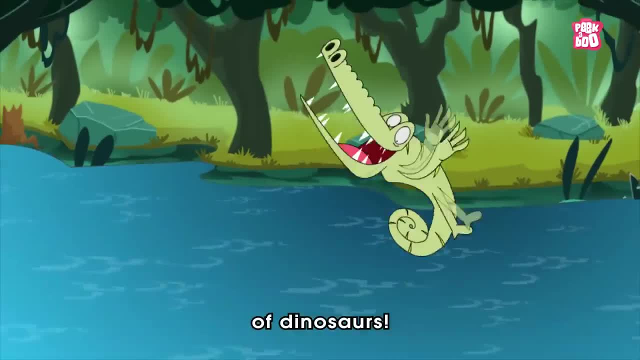 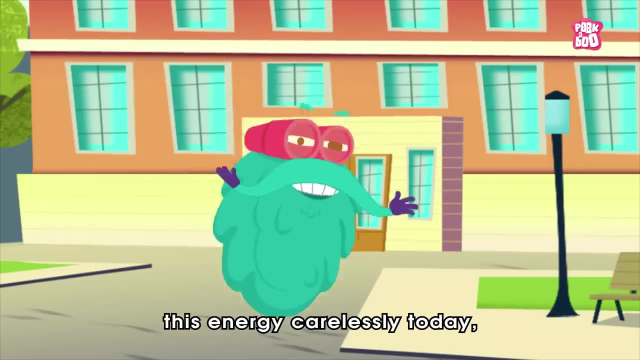 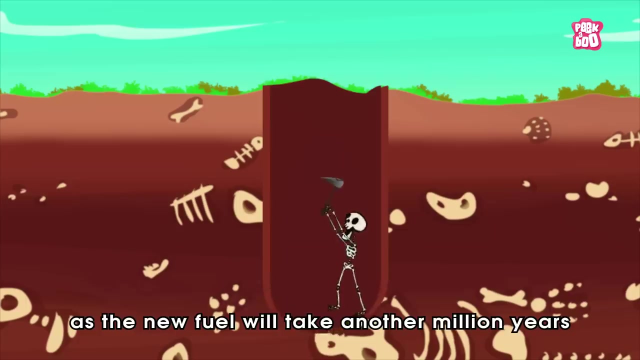 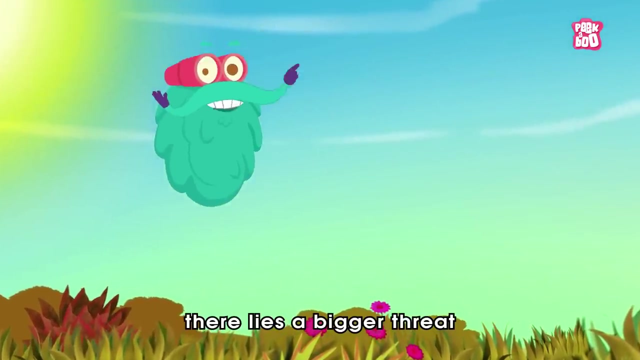 Which is even before the existence of dinosaurs. Yes, therefore, if we use this energy carelessly today, we are going to land into a devastating problem, as the new fuel will take another million years to form again. And apart from this futuristic problem, there lies a bigger threat in the present as well. 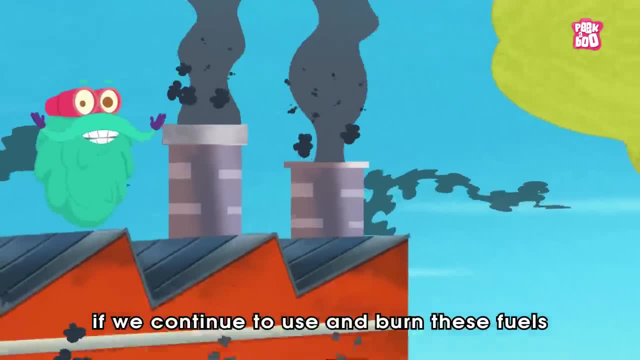 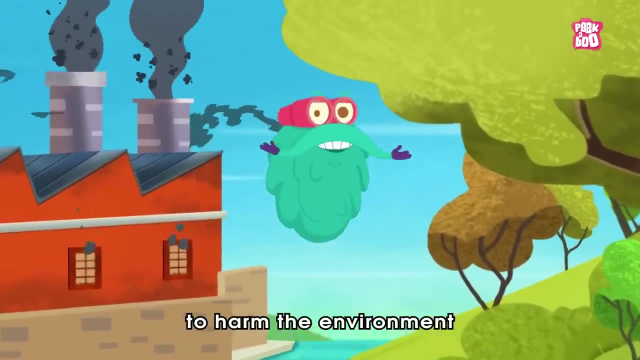 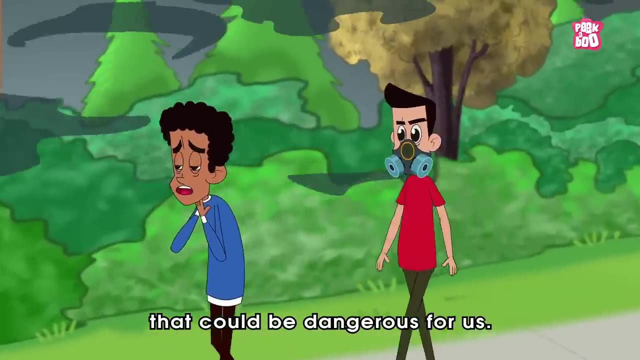 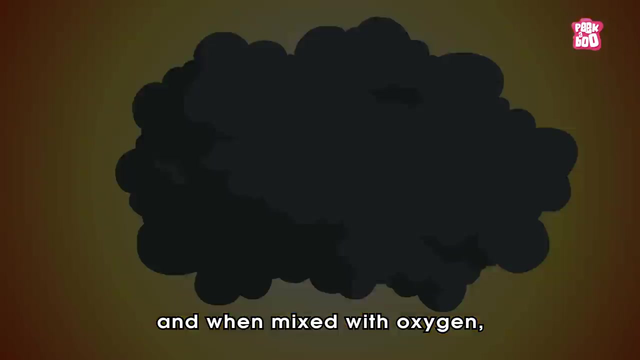 Yes, my dear friends, If we continue to use and burn these fuels at this rate, they also have the potential to harm the environment, as they are made up of harmful chemical bonds that could be dangerous for us. You see, the coal we use is made of carbon and when mixed with oxygen, it leads to an increase in carbon dioxide in the environment. 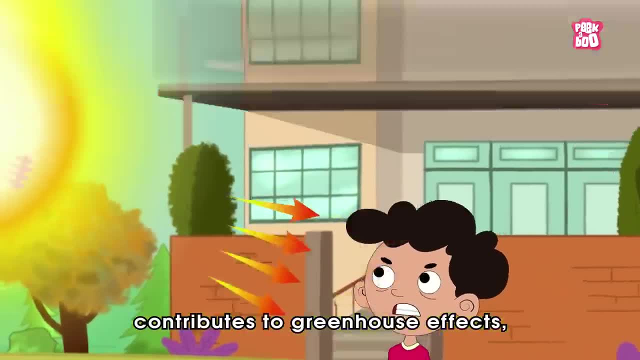 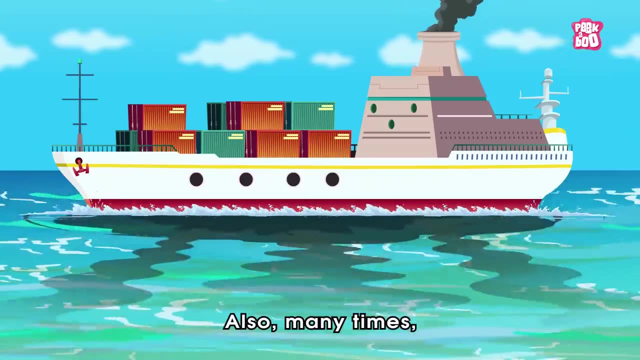 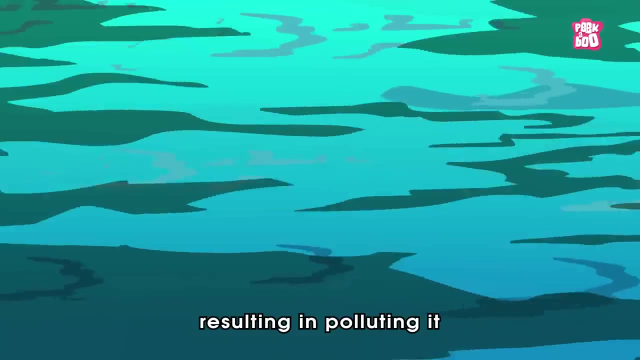 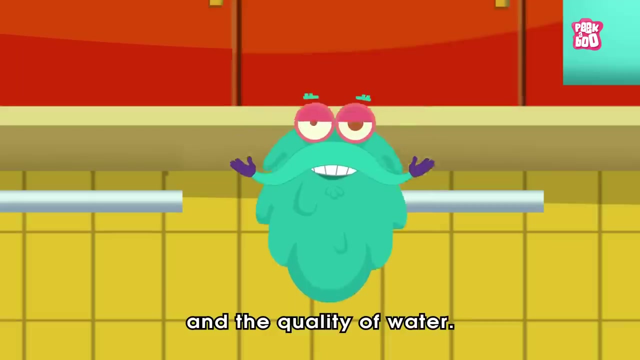 This eventually contributes to greenhouse effects, which then contributes to climate change and cause global warming. Also, many times, the oil spills into the sea during transportation, resulting in polluting it and establishing a threat to all aquatic animals and the quality of water. 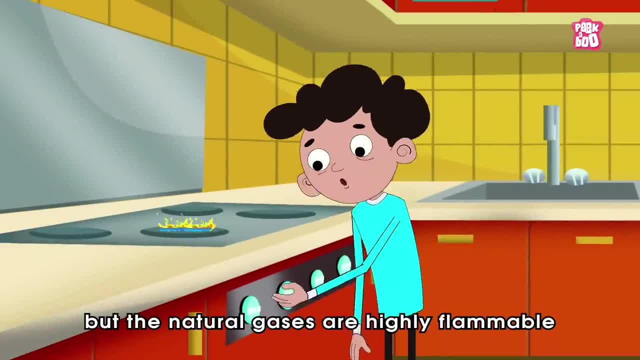 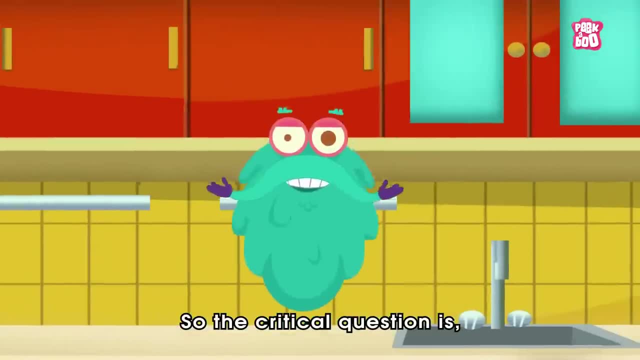 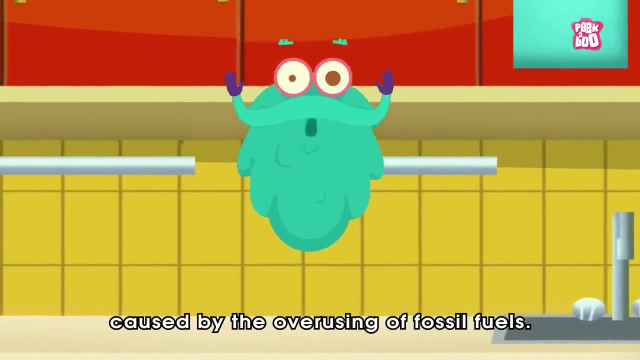 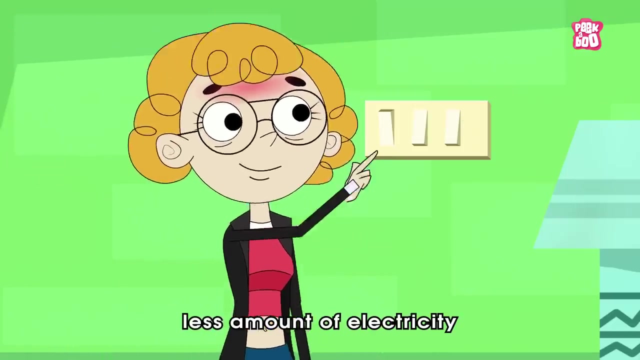 Not only that, but the natural gases are highly flammable That can prove hazardous if not used wisely. So the critical question is: what do we need to do to control the damage caused by the overusing of fossil fuels? Well, we can start by using less amount of electricity, or using it only when required.